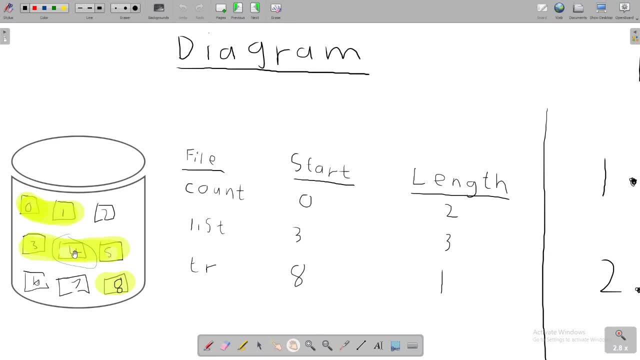 starts counting at zero. so if you don't understand that, I'll just do a small explanation. So because the operating system starts at 0, adding or looking for the second record would be number one, and the reason that is because we start at zero, so zero one. 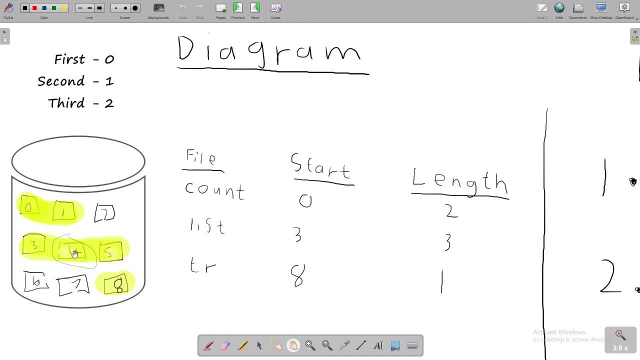 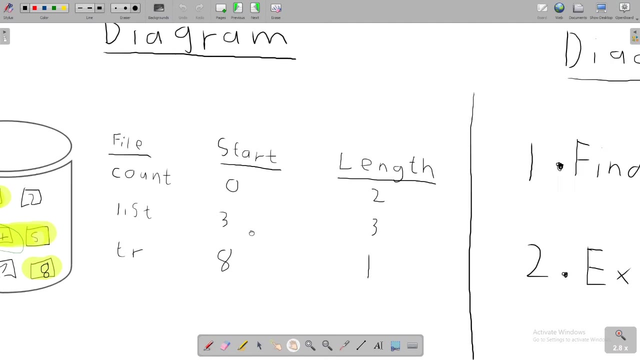 two. now the second one in that count would be one, see zero one. so one would be the second record. so they do three plus one to find the second record in the list file. now this technique does have a few disadvantages, and first off, we run into an issue of finding space for 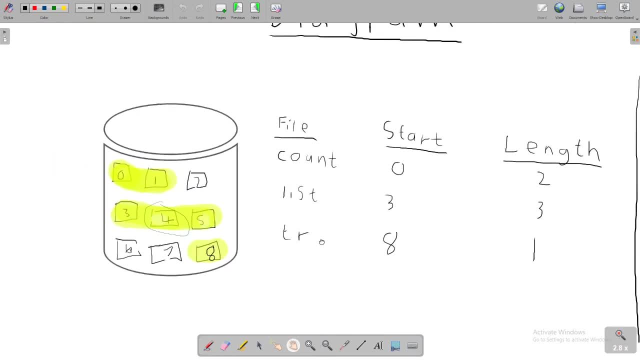 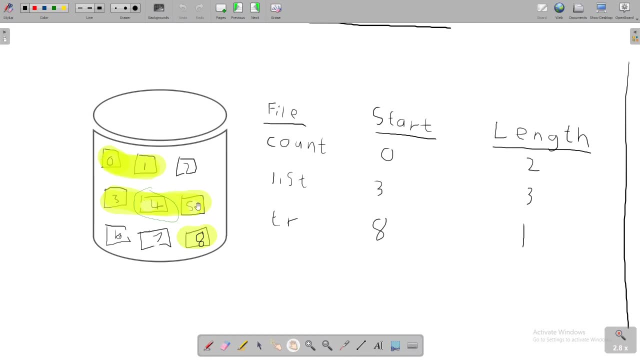 new files. now, if I quickly go back to this diagram, you can notice a pattern occurring here. so if you have a look at these blocks, you will see that they've found enough space and they've been allocated data blocks. but the issue is now: we've got this two sitting. 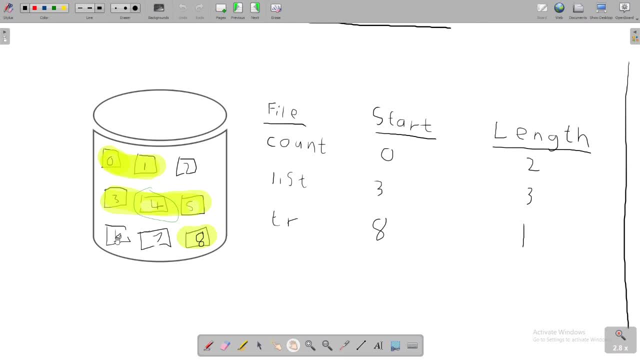 over there on its own, six and seven sitting there on its own. and, yes, if we have files that are two blocks big or one block big, we'll be completely fine. but what happens if we have file that require three to four blocks? then we have an issue where, yes, we might have. 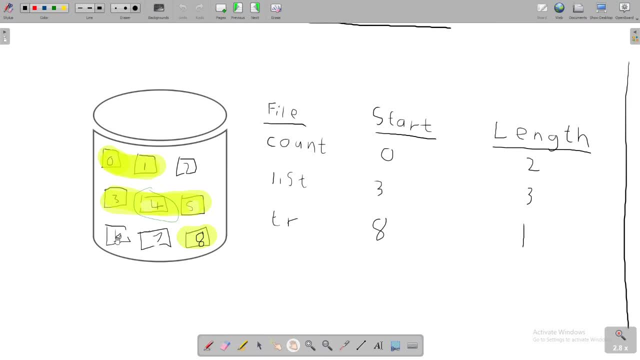 enough space for that file file, but because we're using contiguous allocation technique, it won't allow us to allocate all the space, as those three blocks aren't contiguous with each other. now the second disadvantage we run into is simply external fragmentation, which is essentially what we explained above. 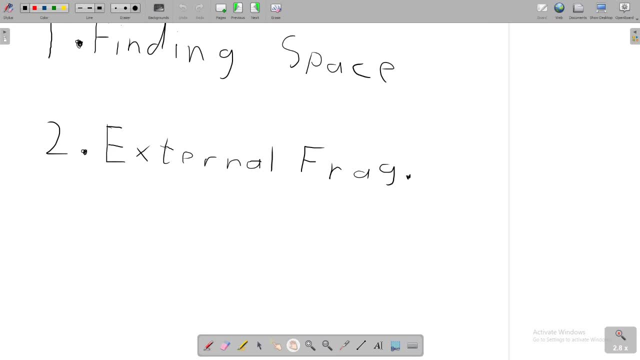 and it's when the total memory space is enough to satisfy our quest. but it is not contiguous, which we know means in sequence. therefore, we can't use it. the next method is to find out where the data blocks are located, which I'll open up here is called linked allocation. 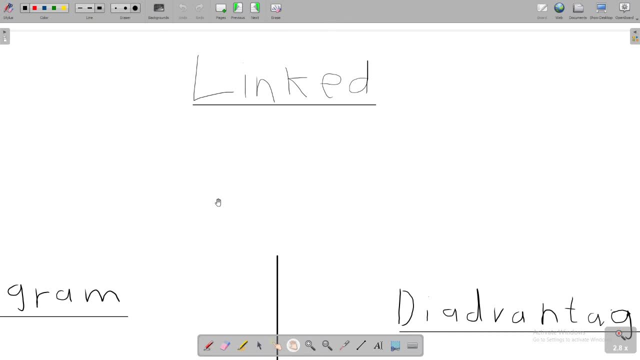 in this file system implementation technique, each file is a linked list of data blocks. now, what that means is that all data blocks are linked to each other. they do not have to be contiguous, which means in sequence or next to each other, but instead can be scattered around. now, due to them being linked, it does not matter where they are placed, and you might. 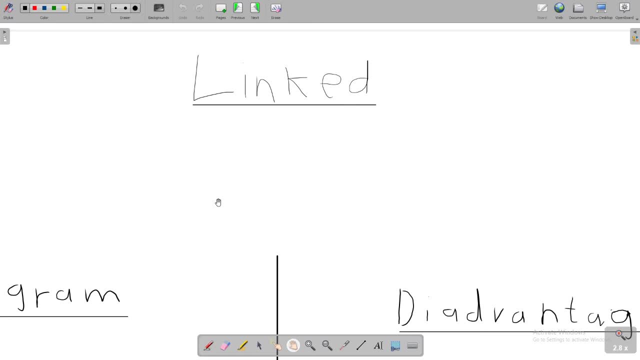 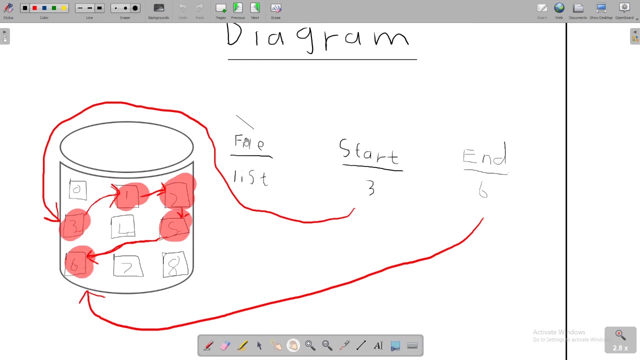 have noticed that this solves the problem of contiguous allocation in terms of external fragmentation and finding space for blocks and finding space as blocks can be scattered anywhere, as they are all linked. here you can see a great example of what linked allocation looks like. the file essentially has a starting point and ending point, which, in our case is: 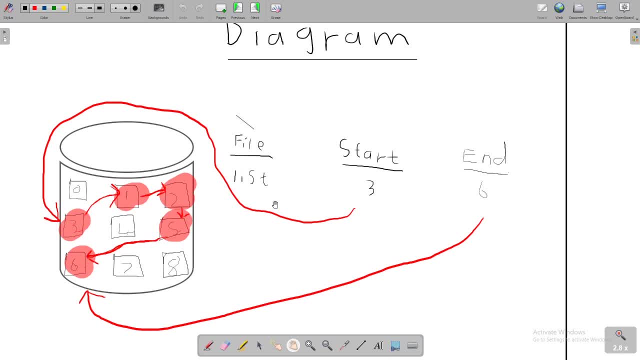 three and six and, as you can see, the order and placing of the blocks do not matter as they are all linked to each other. for the computer to remember what comes after the starting block, a small amount of space is set aside in each block to point to the next and, in some cases, to point to the previous. 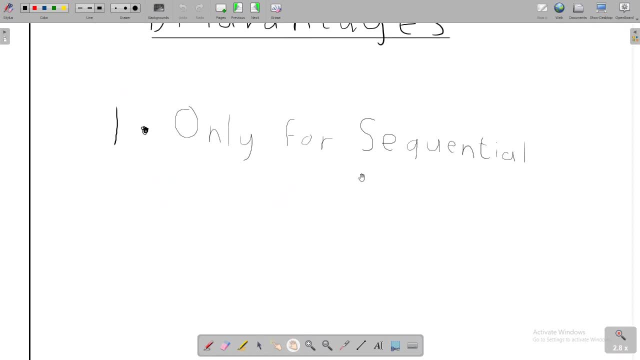 one as well. lastly, it does come with one major disadvantage, and it's only for sequential access. there is no way to use linked allocation and random access, and that's where indexed allocation comes in. now, this is the last technique for allocation. it is known as indexed allocation. 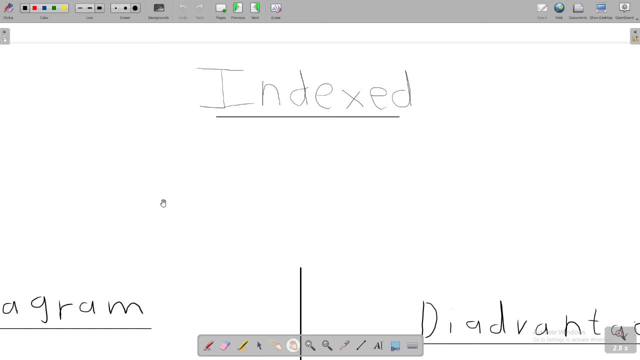 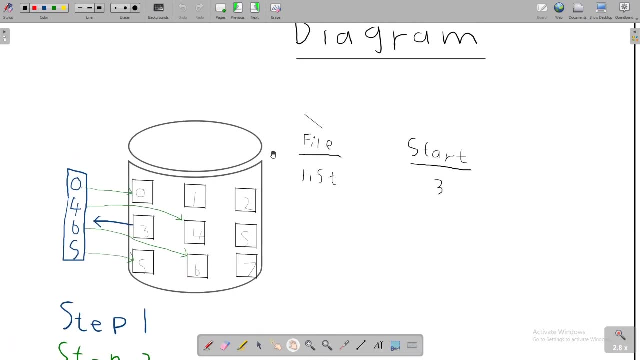 in this technique all the pointers two the other blocks are stored in a single block. this is much better explained using a diagram. in our case we will again use the list file and list starts at block three. in the indexed allocation technique that would mean that the starting block is the block that holds. 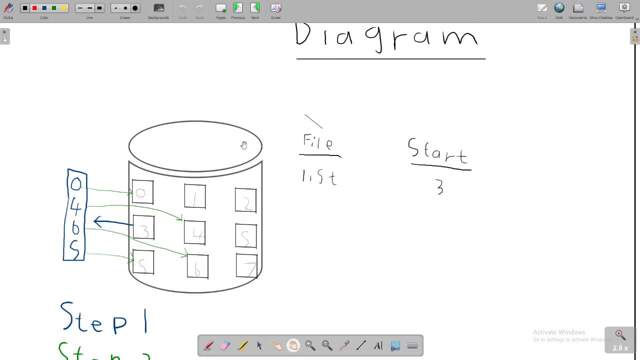 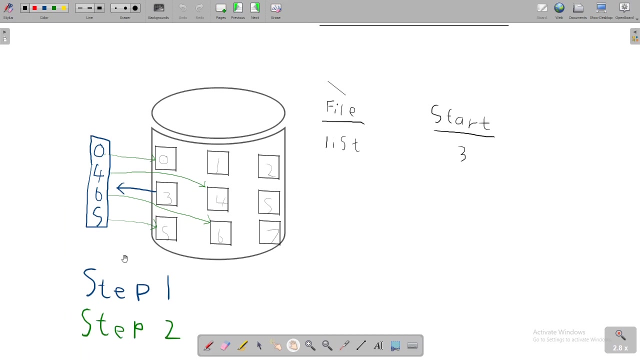 all the pointer information. so if we go to block three we can see here it holds four pointers. these pointers are telling the operating systems that the dotted blocks that occupy the files are in those locations. the first dotted block for the list file is zero, then four, then six and so on, as you see below. i. 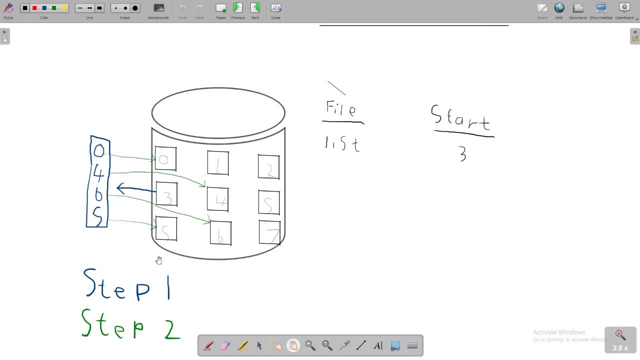 have written the steps the os takes to access the block. first, it goes to the indexed blocks and finds all the pointers, and second, it goes to the pointed locations to access the blocks. now this solves the issue of external fracturing. This is because it's supporting direct access to the blocks occupied by the file and on.